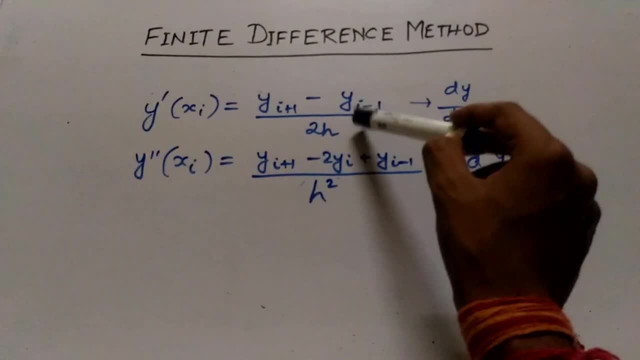 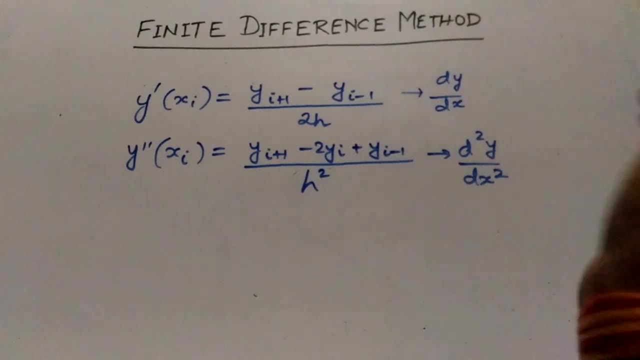 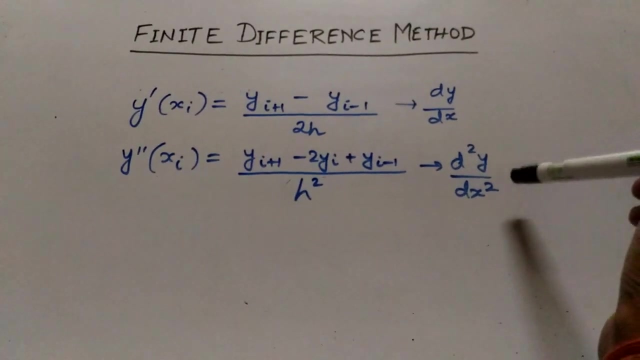 is 1, then you have to replace it by this expression: that is yi plus 1 minus yi minus 1, divided by 2H. Similarly, if the notation is in the order of 2, that is second order derivative. if it is given, that is d2y d medieval. 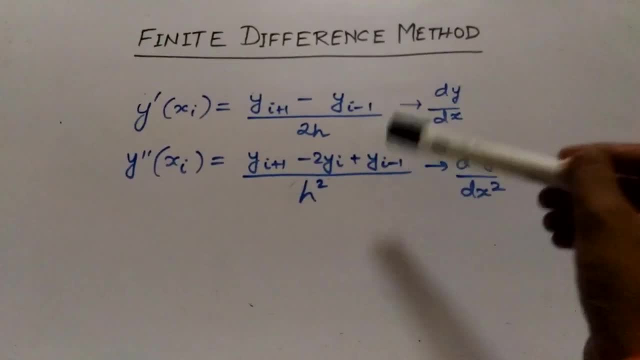 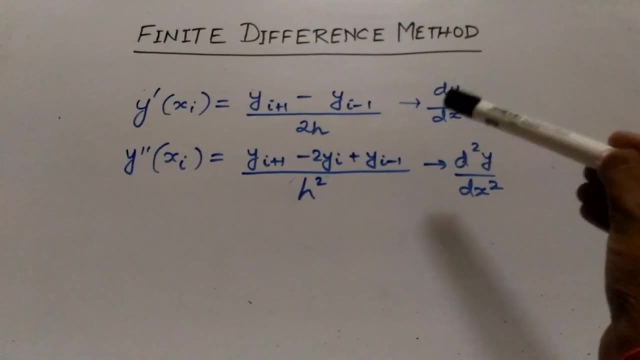 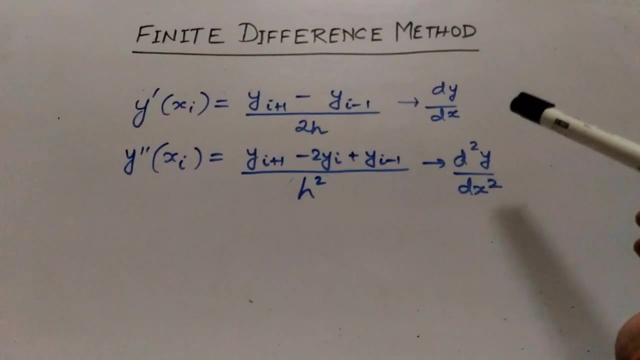 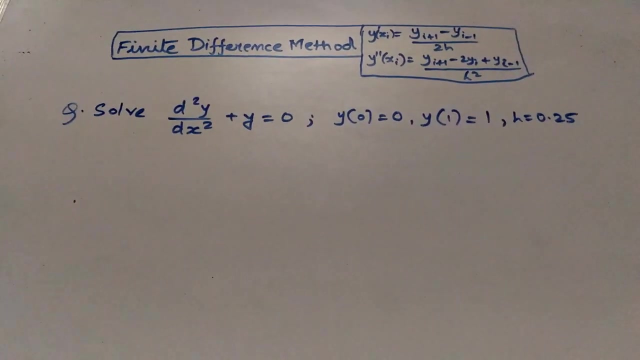 2, then you have to replace it by this expression, that is, y i plus 1 minus 2, y i plus y i minus 1 divided by h square. So you have to keep these two expressions in mind before proceeding with the finite difference method. Now let us look at the example to understand the finite. 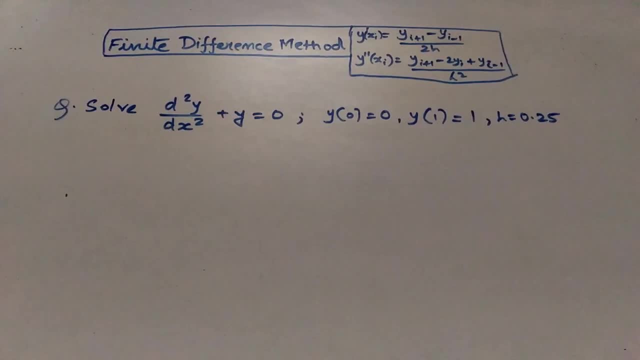 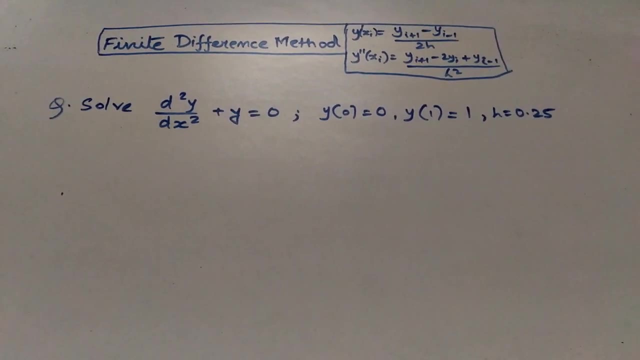 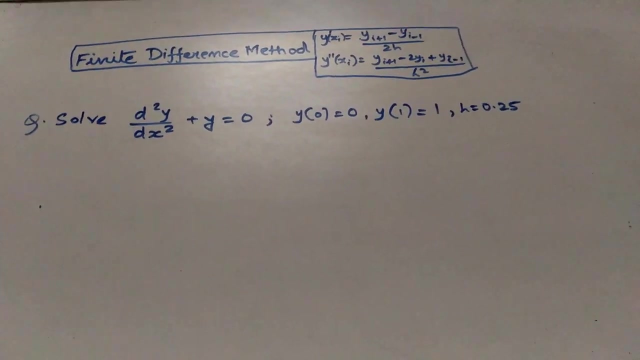 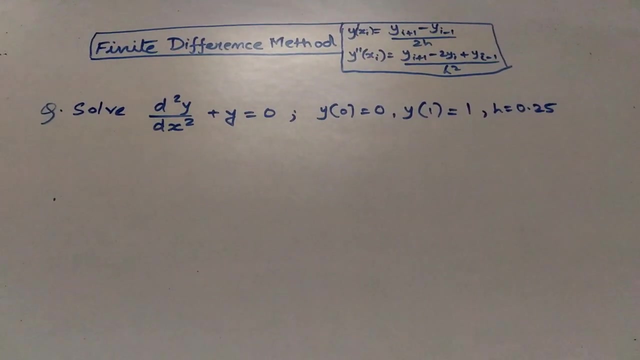 difference method. The question is: solve d2y. dx2 plus y equals to 0.. Our boundary conditions are: y equals to 0 when x equals to 0 and y equals to 1 when x equals to 1 and the value of h has been given, that is, 0.25.. Now our first task will be to replace the differential. 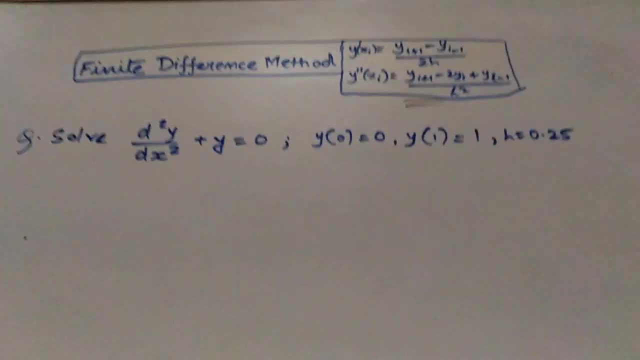 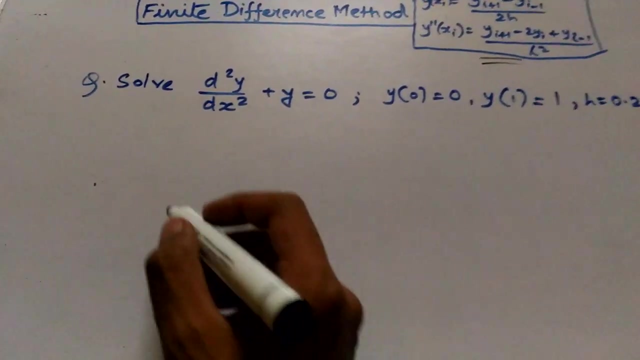 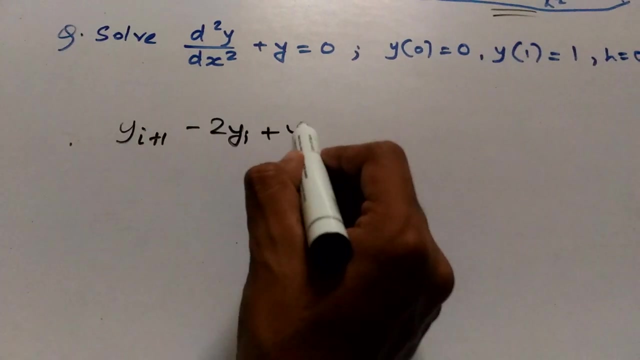 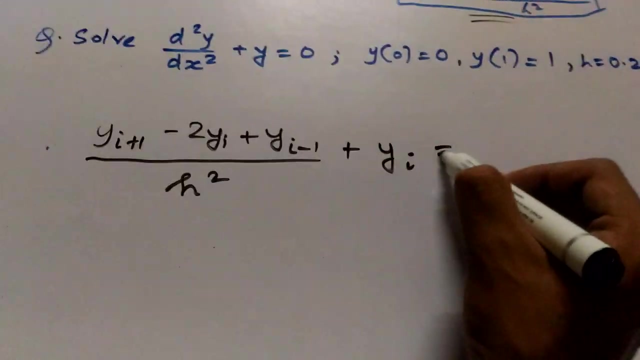 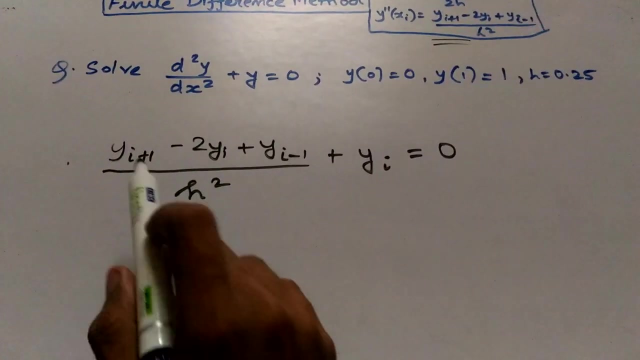 notation by this expression. So I will rewrite the differential equation in the form of y i. So it will be y i plus 1 minus 2, y i plus y i minus 1, divided by h square plus y i is equal to 0.. Now I will make this: 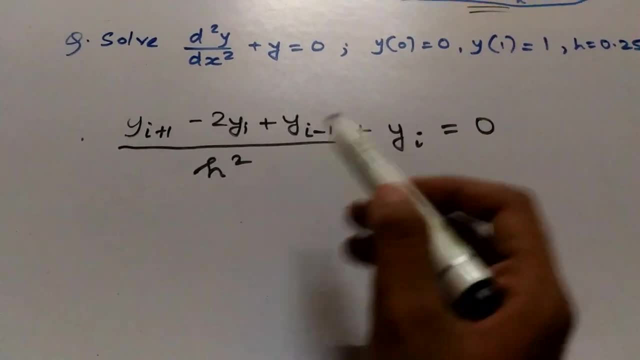 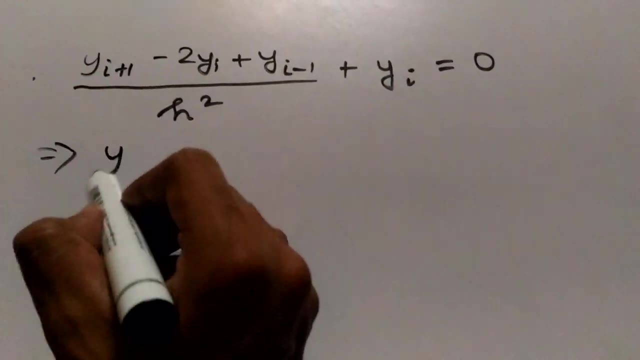 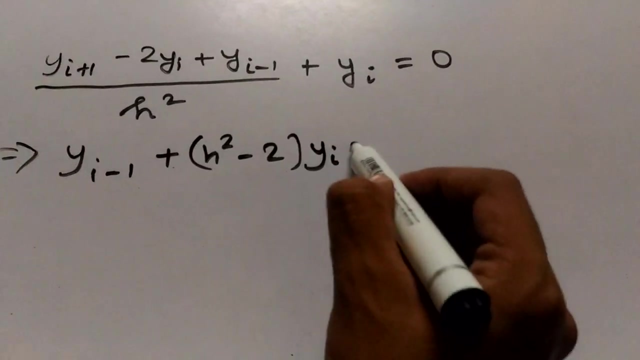 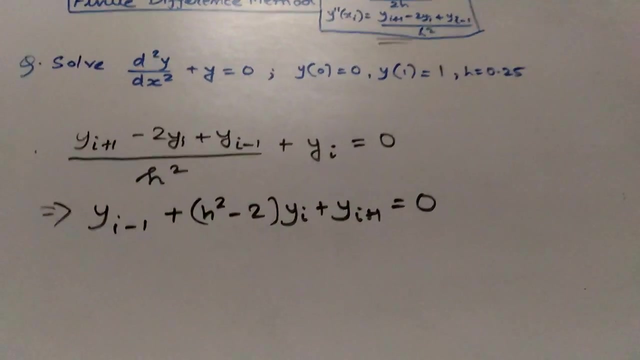 equation linear by multiplying h square. So I will write the equation with y, i and 0.. Therefore our equation will become y i minus 1 plus h square minus 2 into y i plus y i plus 1 equals to 0.. So this is our equation. 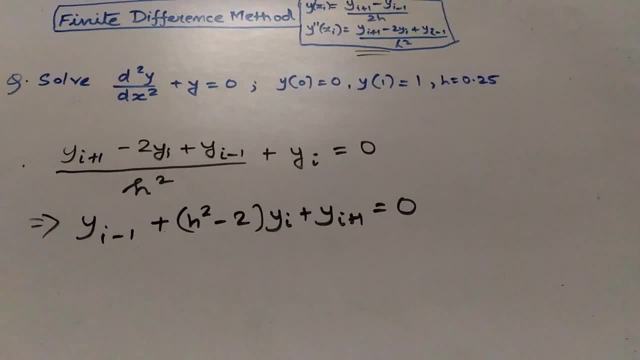 Now what I will do. Now, I will put the value of h. This is the equation Now. I will put the value of h. Now, I will put the value of h. This will be the equation. Now, what I will do is I will. 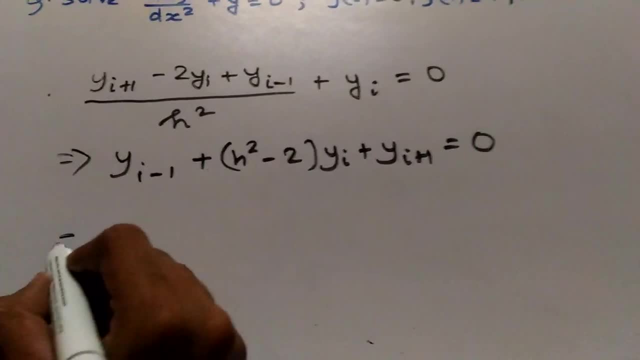 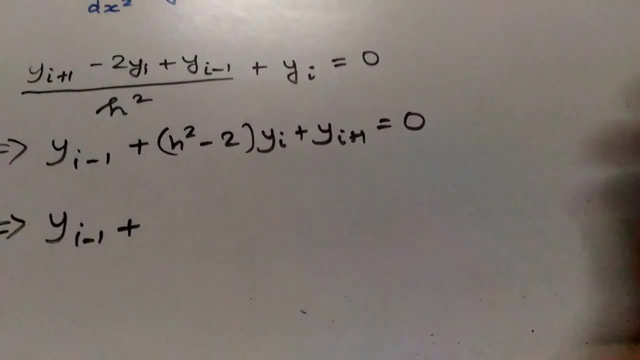 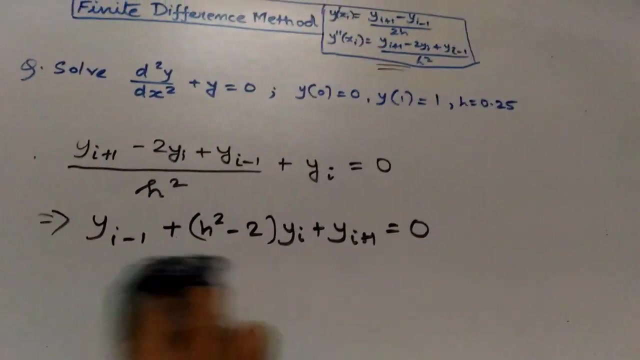 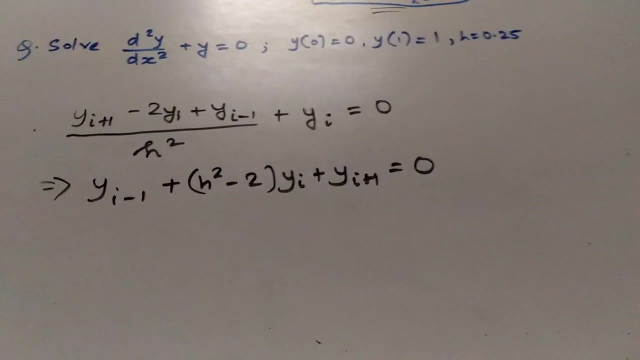 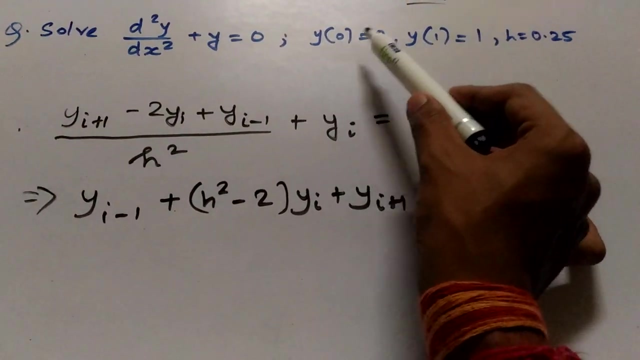 h in this equation and then I will get the final equation as y i minus 1 plus sorry, first of all, I will put the values of i here. Now, what I will, what I, what values of i I will put, since the boundary condition is x equals to 0 and x equals to 1. therefore, and and also: 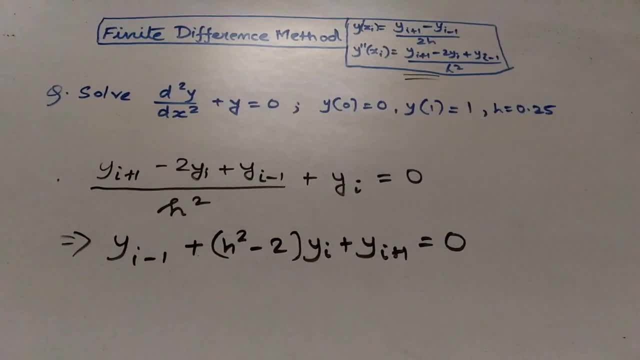 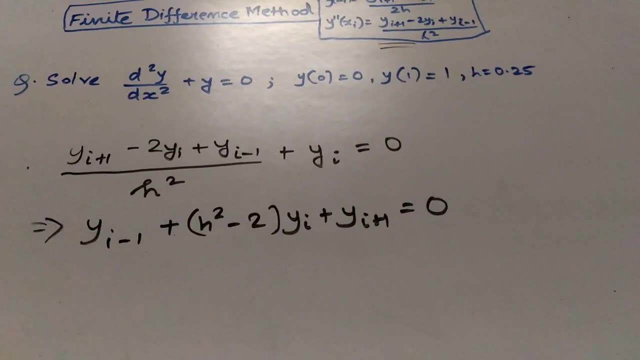 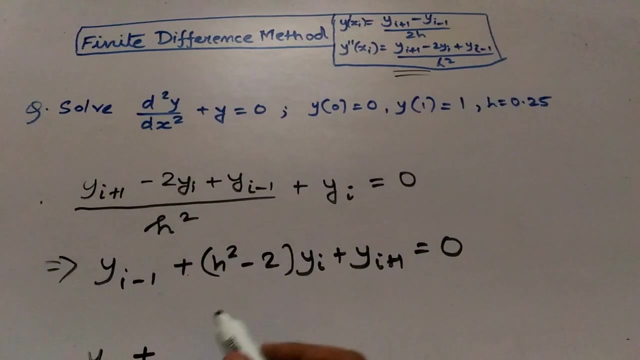 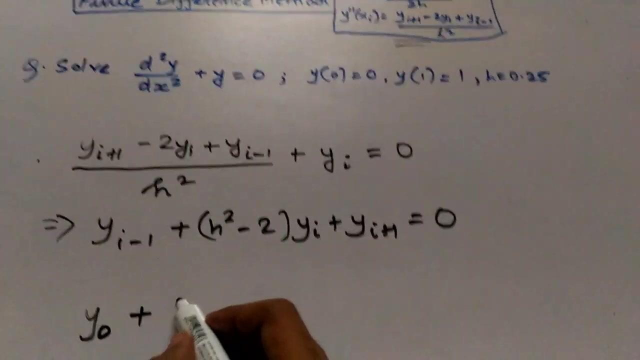 our h is 0.25. therefore i will be i. the values of i will range from 0 to 3.. So our y i minus 1 will be 0. y 0 plus I will put the value of h here, So it will become h. square means 0.25 square minus 2. that is one point that will be minus. 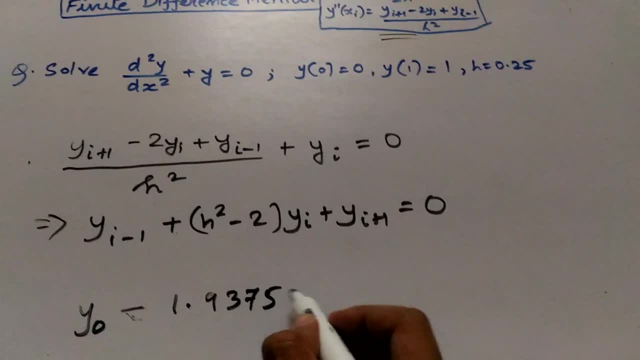 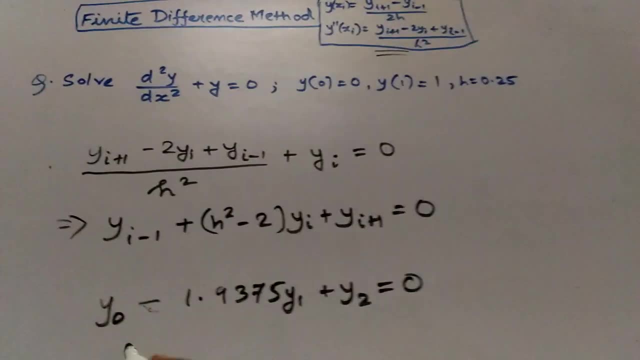 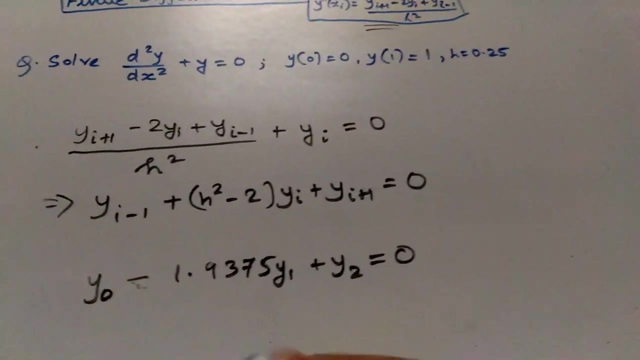 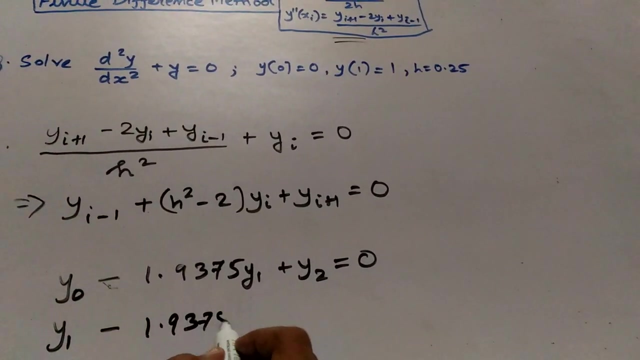 minus 1.9375 y1 plus y2 equals to 0.. Then I will move on to the next value of i, that is, i minus 1 will be 1. therefore, y1 minus this will again remain same. 1.9375 y2 plus this will be y3 equals to 0.. Similarly, the next. 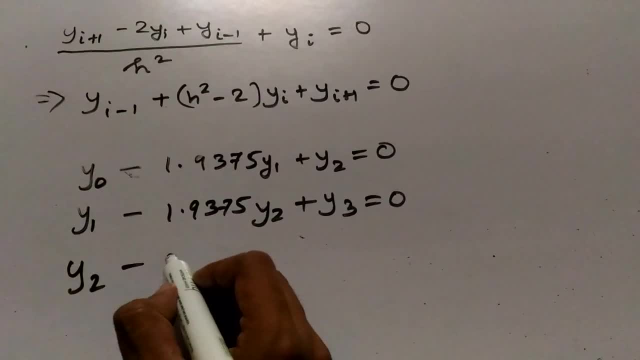 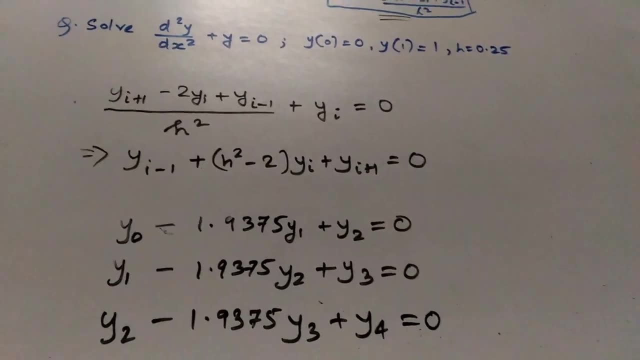 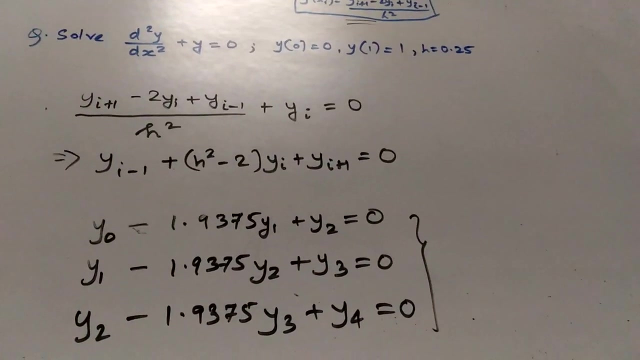 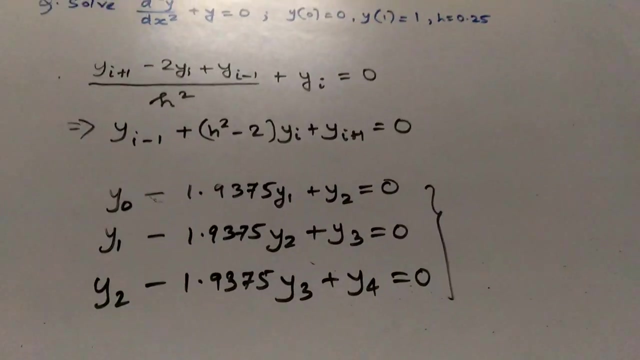 equation will be y2 minus 1.9375. y3 plus y4 will be equal to 0.. So this is our system of linear equations. This you can solve by any method. you can solve it by substitution method, you can solve it by cross multiplication or you can solve it by the. 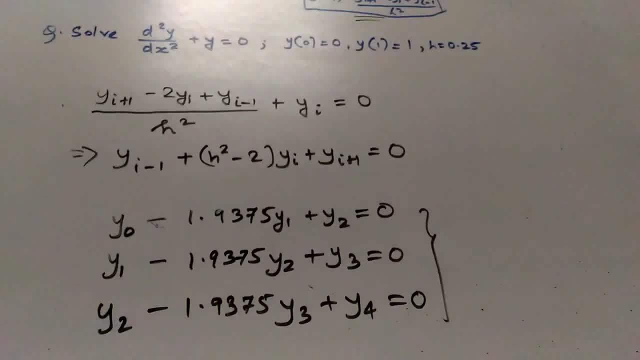 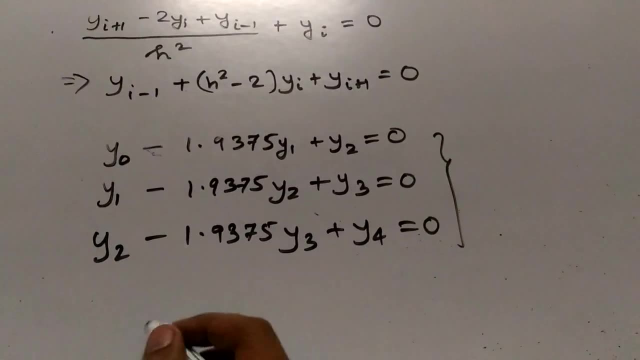 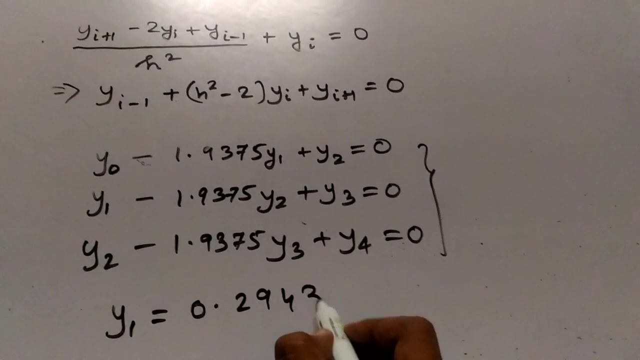 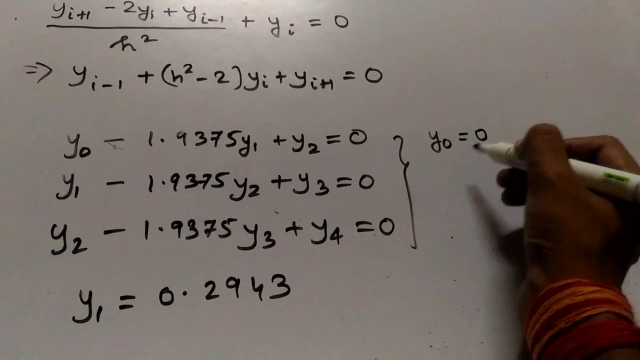 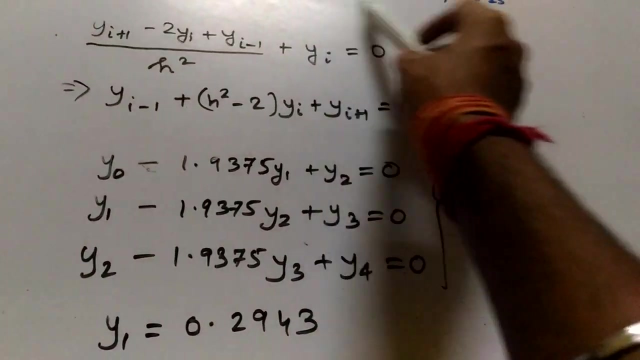 gauss, elimination, matrix, inversion, LU, factorization, any method you like. So, on solving these three equations, I will get y1 as 0.2943.. Now, before that, I must tell you here: our y0 is nothing but 0. And our y4 is nothing but 1, since our boundary conditions. you can see, y0 is 0 and y4 is 1.. 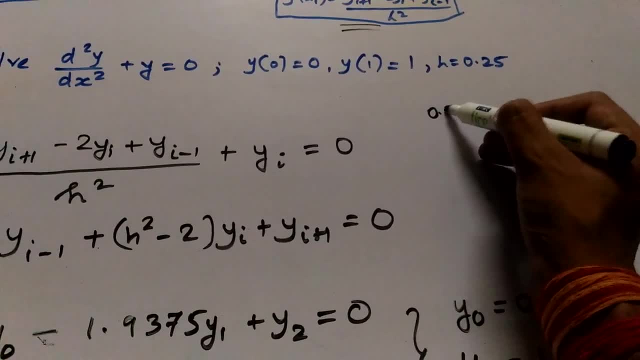 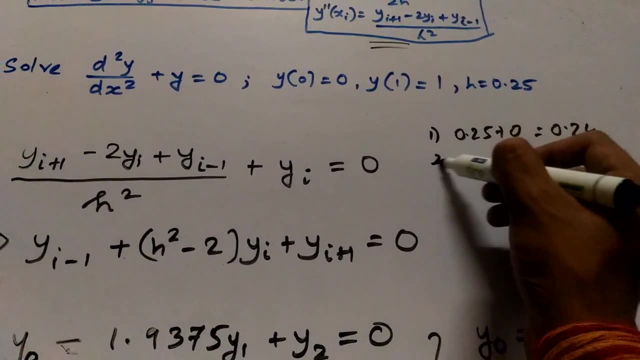 Why y4 one? because adding 0.25 to 0. We will get 0.25. this is the first one. second 0.25 plus again 0.25.. We will get 0.5.. That's 0.25, 2.5.. 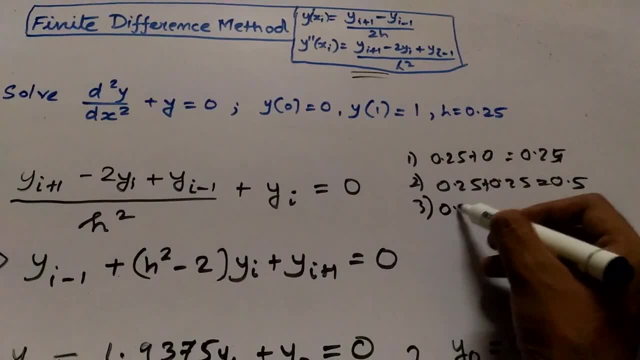 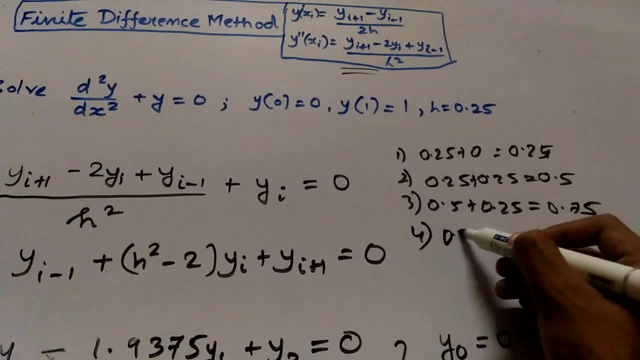 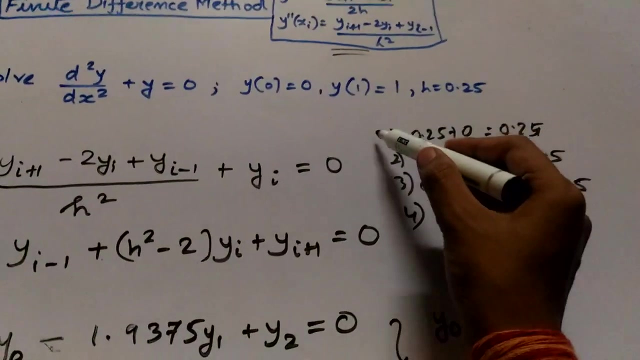 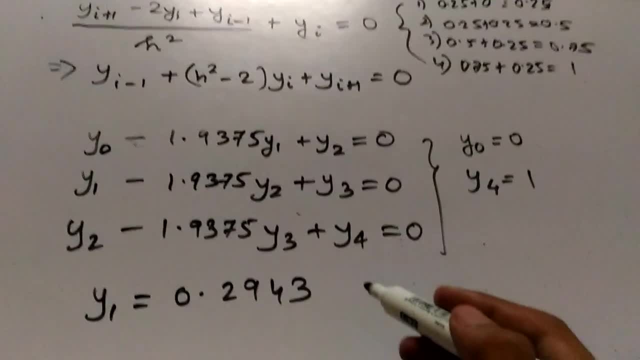 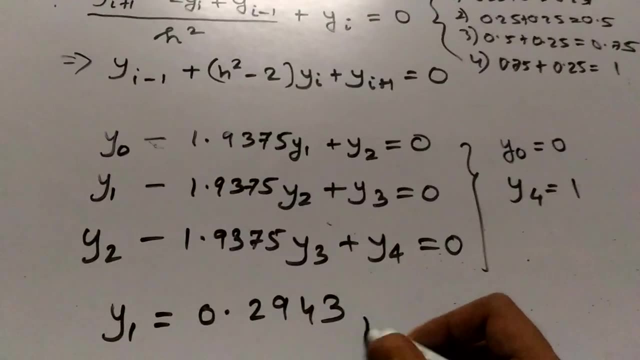 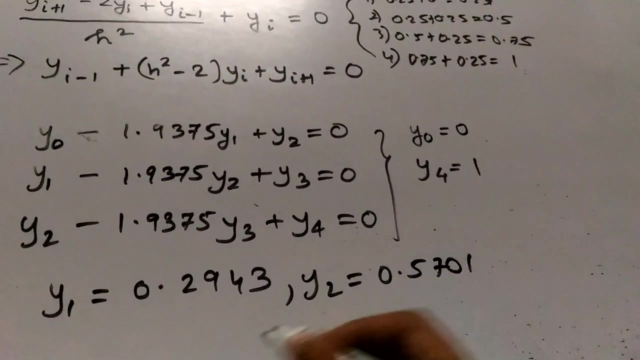 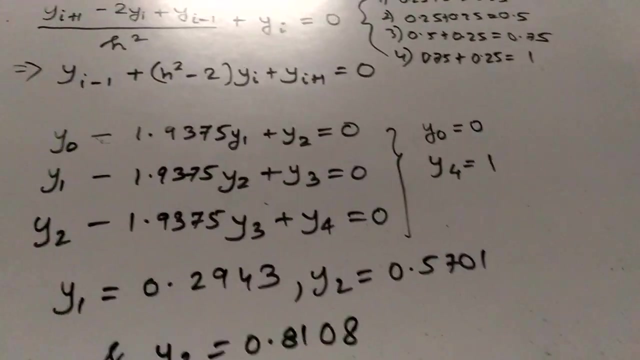 equals to 4. therefore y4 is 1. so, putting these values, we can solve the equations very easily. now we will get y1 as 0.2943, y2 as 0.5701 and y3 is 0.8108. so we will get our values. we. 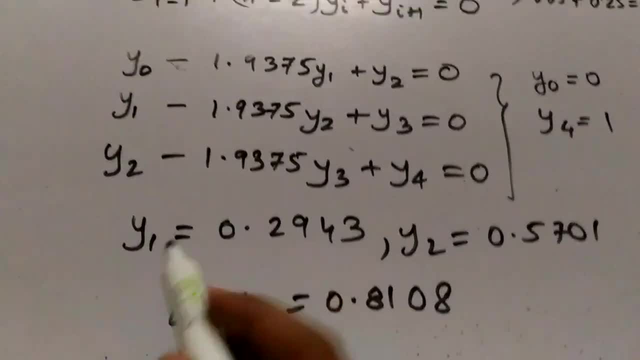 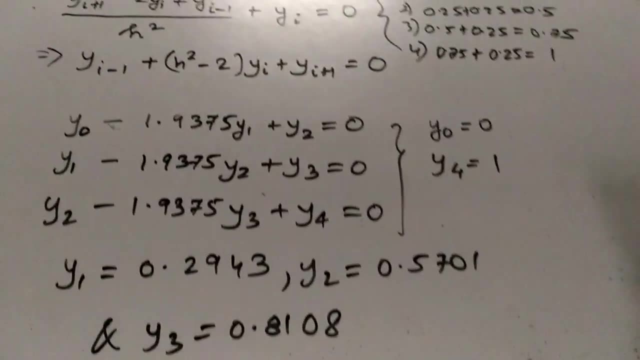 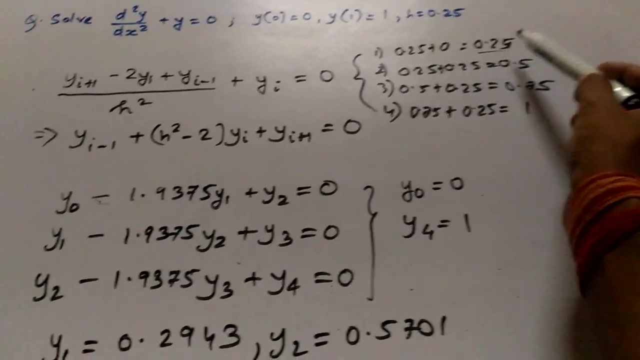 can. we will get all the values. so y1 means 0.. y1 means is y 0.25, y1 is 0.25. y2 means y 0.5. that is the values of x. the values of y at 0.25 is nothing but. 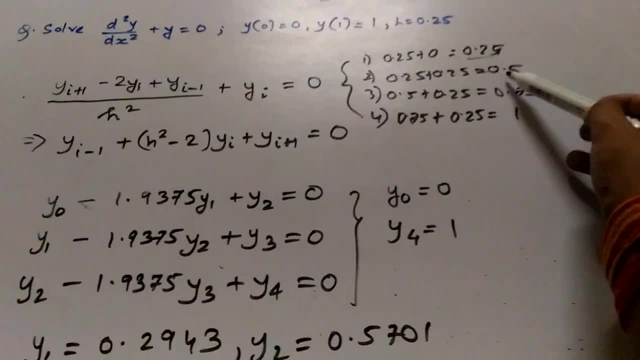 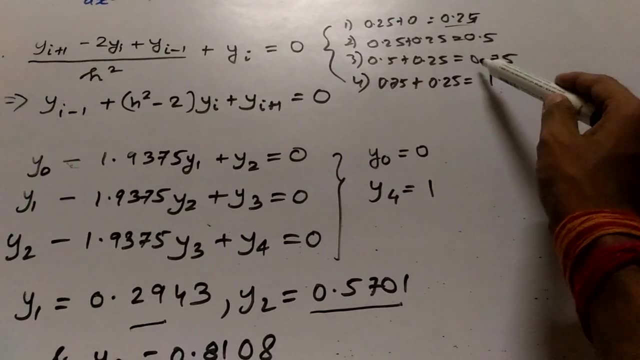 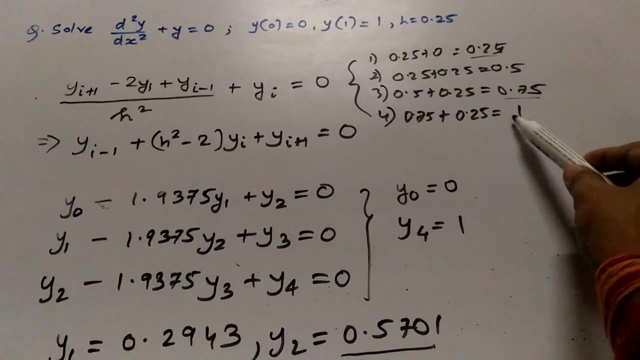 0.2943. the value of y at x equals to 0.5. it is nothing but 0.5701. the value of y at x equals to 0.75 is nothing but 0.8108, and we know. the value of y at x equals to 1. it is also 1. 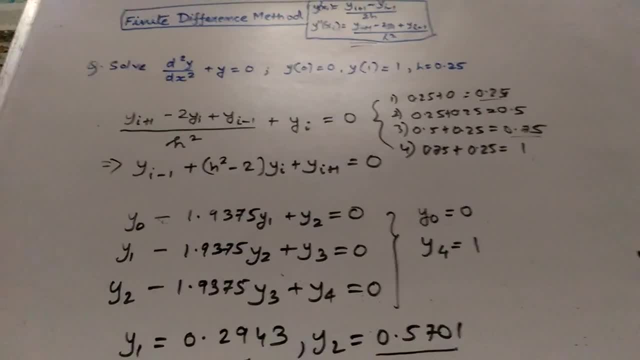 so this was how we can solve differential equation using the finite difference method. thank you.